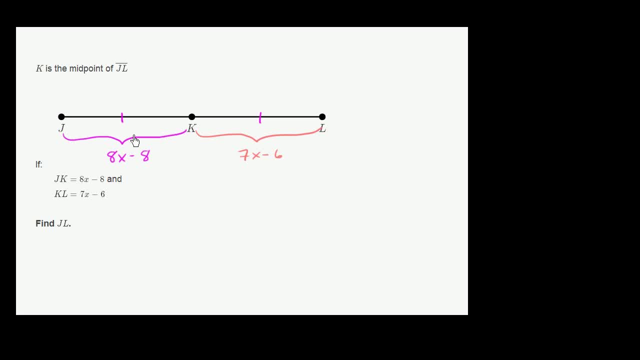 to know what this length is and what this length is. And we could either double one of them or add them together to find the length of the entire segment. So first let's figure out x. And the best way to figure out x 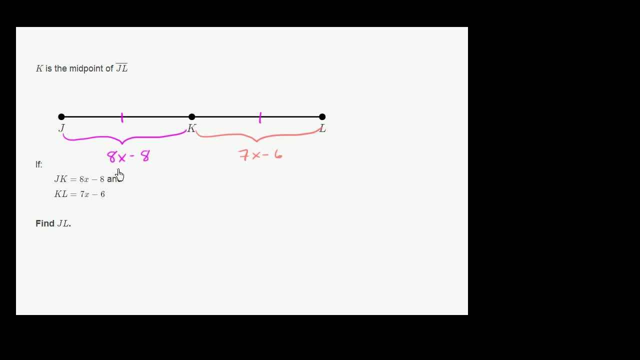 is based on the fact that we know that 8x minus 8 is equal to 7x minus 6.. And I just want to re-emphasize: how do we know that? Well, they told us that k is the midpoint of JL. 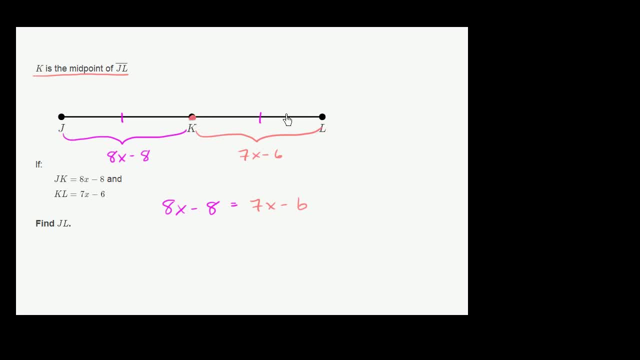 This is the midpoint, which tells us that this distance is equal to this distance, Or 8x minus 8 is equal to 7x minus 6.. Now to figure out x, we just have to do a little bit of algebra. 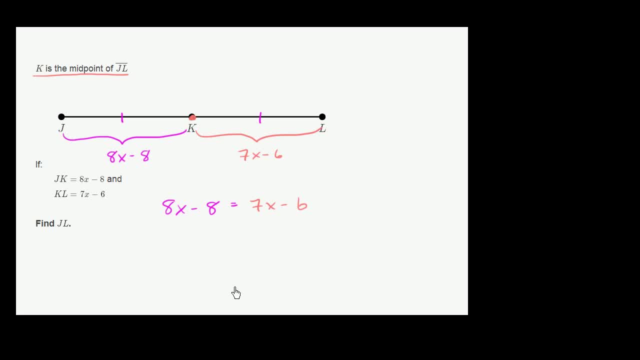 So let's see what we can do to simplify things. So if we want to get all the x terms on one side- let's say we're going in on the left side- we could subtract 7x from both sides, So let's do that. 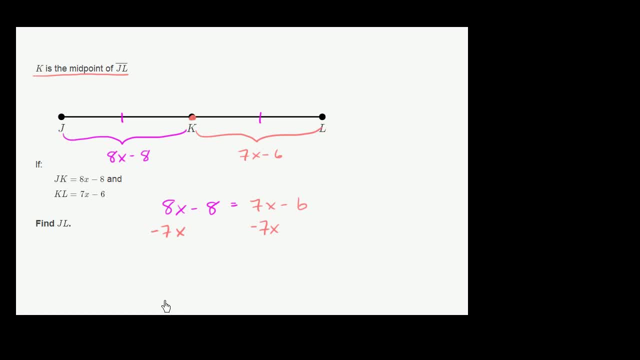 Let's subtract 7x from both sides And if we want to get all of the constant terms on one side, well, let's add 8 to both sides so that we don't have this negative 8 right over here. So let's add 8 to both sides. 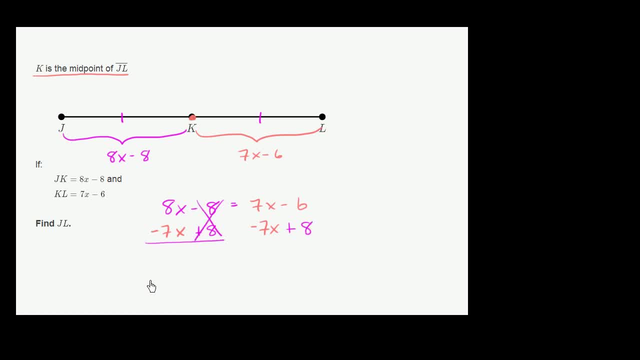 And let's see what we are left with. On the left-hand side, you don't have an 8 anymore. An 8x minus 7x is just an x, And that's going to be equal to. on the right-hand side, 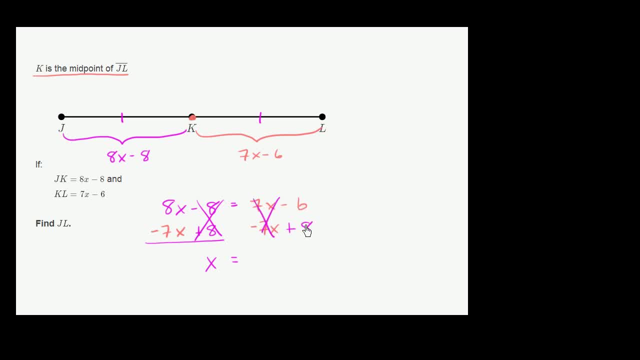 you don't have any 7x's anymore And negative 6 plus 8 is just 2.. So we get x is equal to 2.. But we're not done yet. They didn't say solve for x, They said find JL. 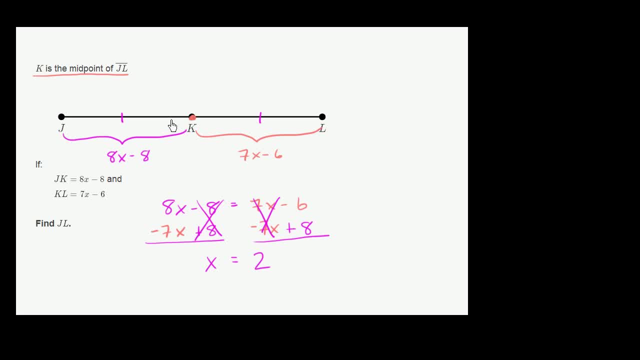 So JL is just going to be the sum of JK and KL, Or since k is the midpoint, it would just be double JK or double KL. So let's figure out either way. So now we can figure out that JK the length of segment JK. 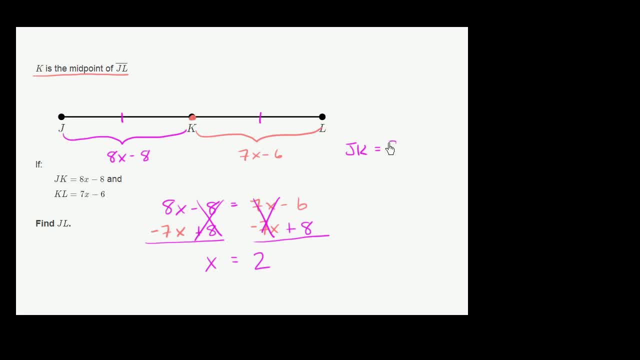 is equal to 8 times 2 minus 8.. We know that x is 2 now, So this is equal to well. this is 16 minus 8.. This is just equal to this right over here is just equal to 8..